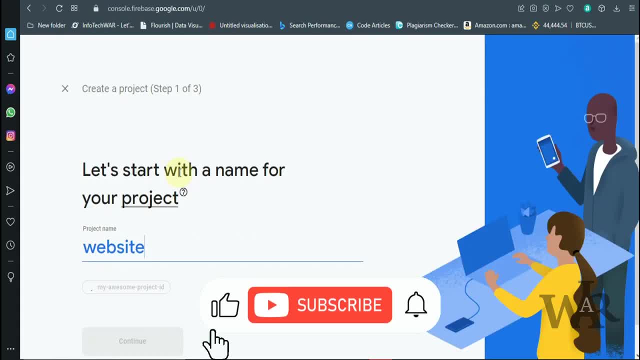 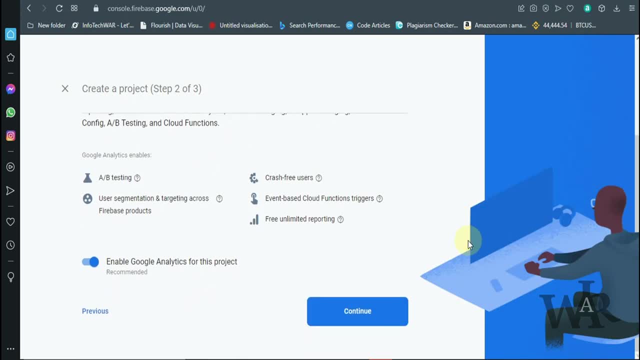 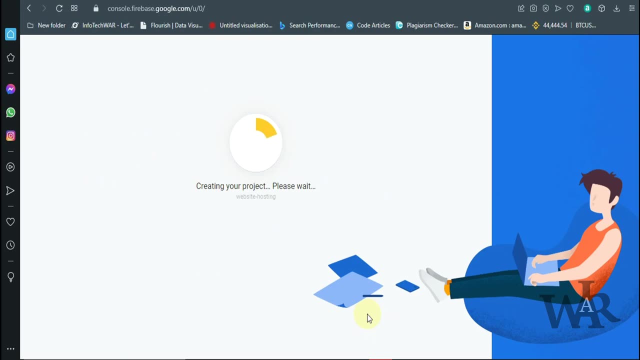 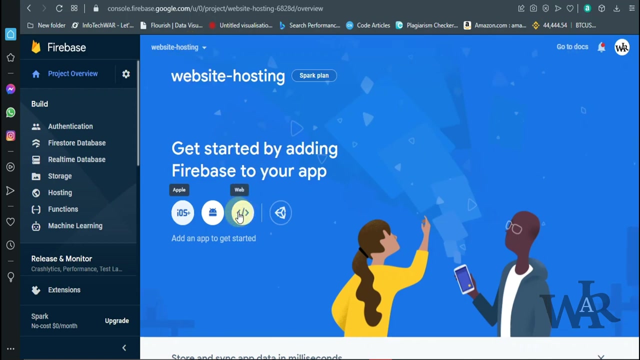 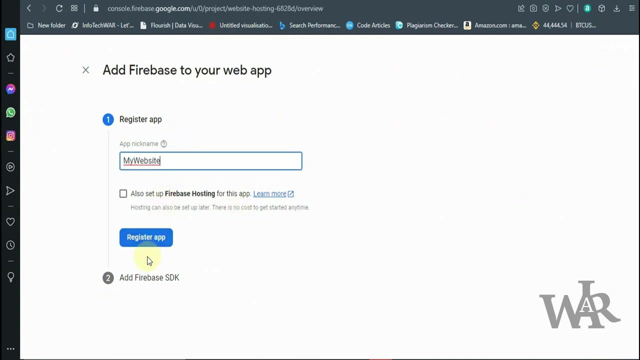 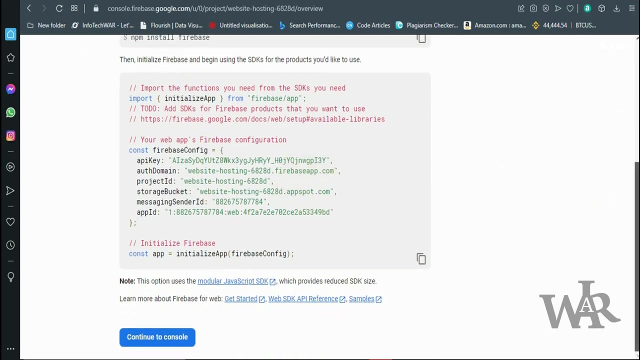 project. give a good name. if you need Google Analytics for your project, you can enable this switch. perfect, now I'm gonna create a new web application. good name for our application. we will set up firebase hosting later. for the time being, we don't need these configurations. I'm gonna go ahead and continue. okay, now we 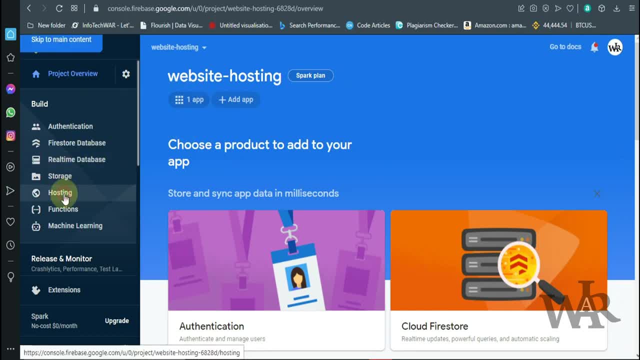 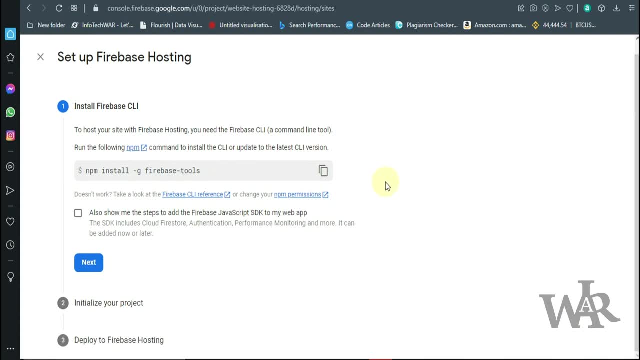 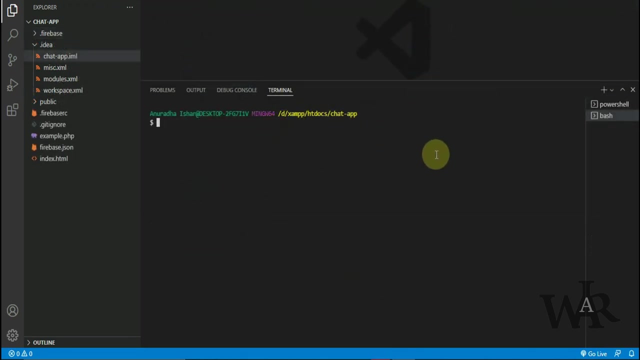 need to create a new web application, so I'm gonna create a new web application. have created our application, which means now we can set up hosting. so now it is asking us to install firebase CLI. so just copy this command and open your terminal. go to the application that you are going to host. for this process you 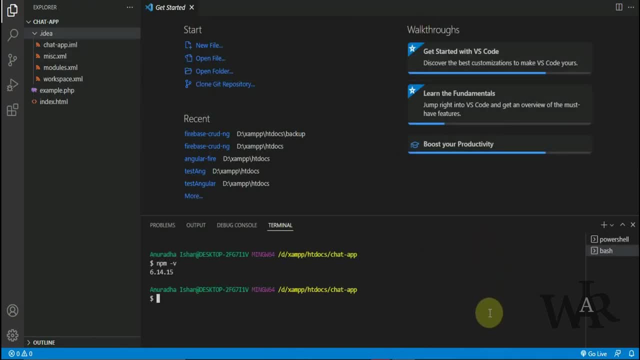 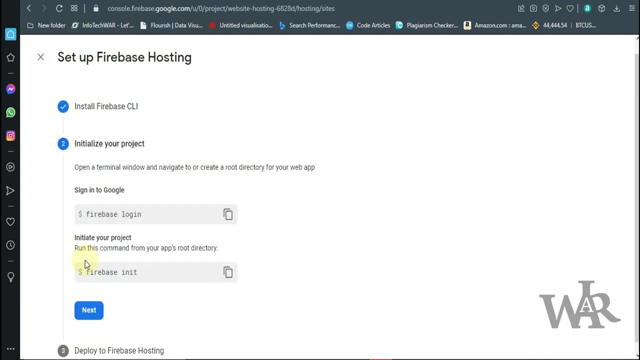 need to install nodejs, so I have already installed it. I'm gonna paste the command line and run it. great, now I have installed firebase CLI and let's go to next process. now it is asking us to initialize our project. first we need to log into firebase using the terminal. 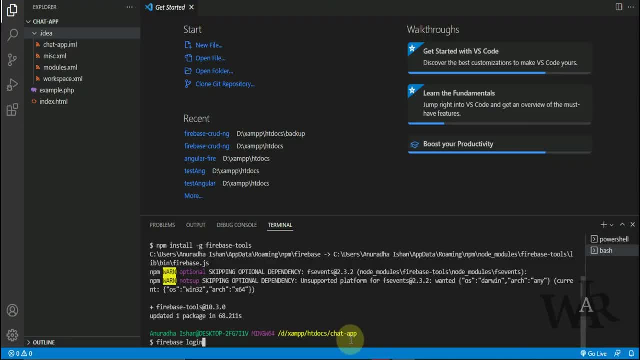 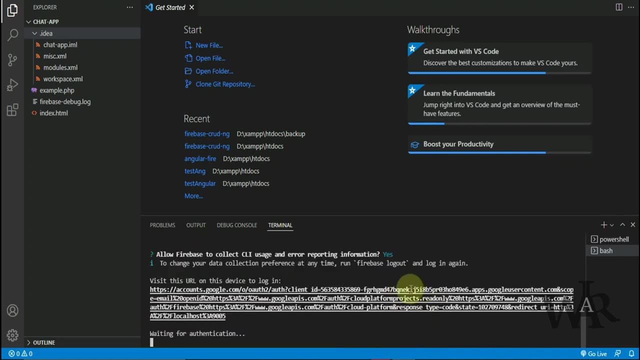 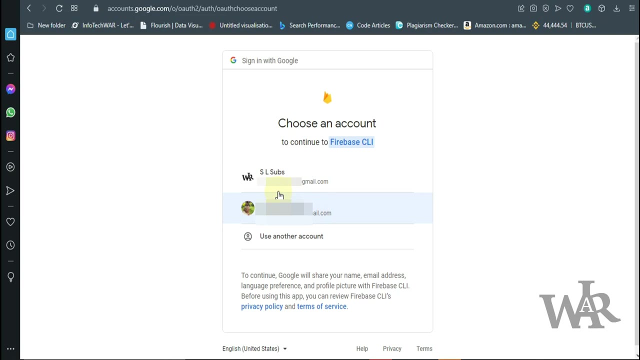 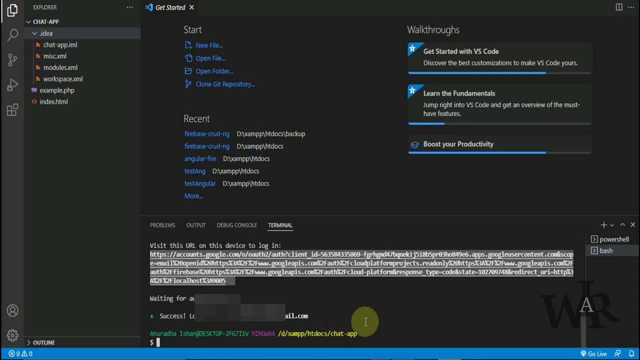 just copy this code and paste it on the terminal. now it is asking us to log into firebase using this URL. just open this URL. so here we have to select one of our gmail account. allow the permissions. now we have successfully logged into firebase CLI, let's go to next step. now we have to initiate our project. 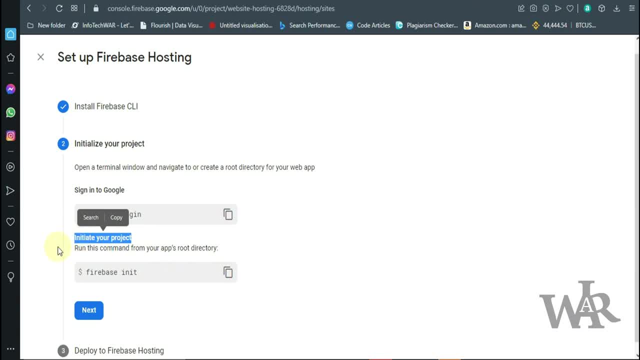 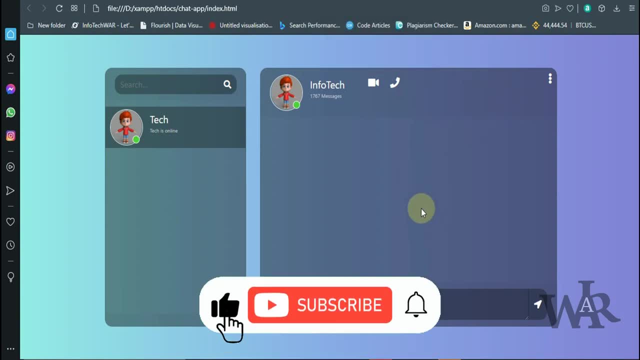 so before that, I'll show my application that I'm going to host. this is a chat application created with firebase real-time database. we created this application in the previous video. if you need to create this kind of chat application, follow my previous video. I'll add the link in the description.